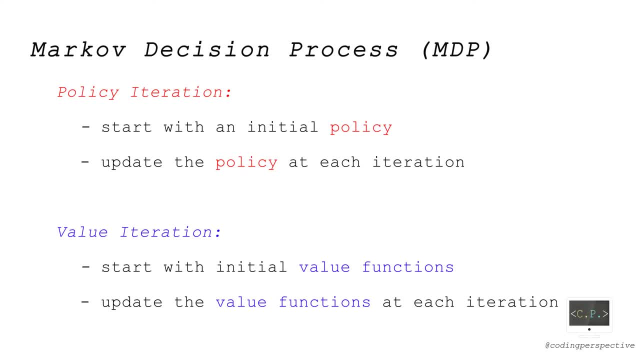 the value iteration algorithm. starting with initial value functions, we find the optimal value functions by iteratively updating them until they converge. This is the main difference between these two algorithms. The policy iteration is an iterative algorithm and consists of three steps. In the first step, we initialize a policy pi 0, with some feasible actions. Then at n iteration i, pi i denotes some possible actions. In the third step we initialize a policy. pi 0 with some feasible actions. Then at n iteration i, pi i denotes some possible actions. In the third step we initialize a policy. pi i denotes some possible actions. 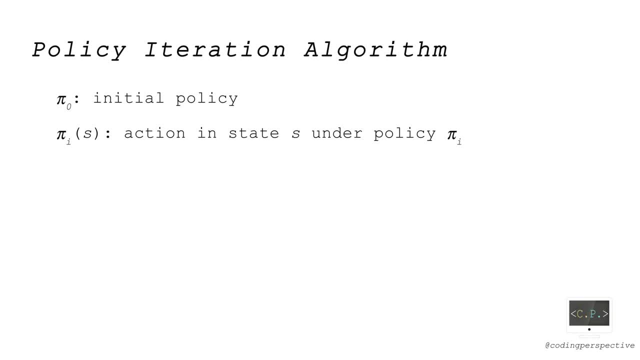 Then at n, iteration i, pi i denotes some possible actions. Then we define v-pi as the expected reward or the value function in state S under policy pi i. We can calculate v-pi by taking action pi as you see for each state S. 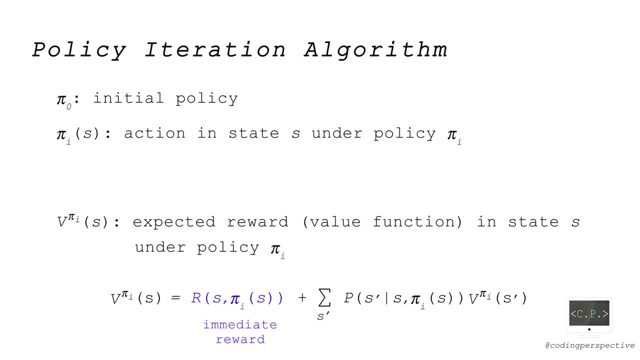 On the right-hand side. the first part of the summation is the intermediate reward and the second part is the expected future reward. i appears in both sides of the equation. Here we have a coordinate offset as different linear equations to solve so that we can calculate the value functions under policy pi i. 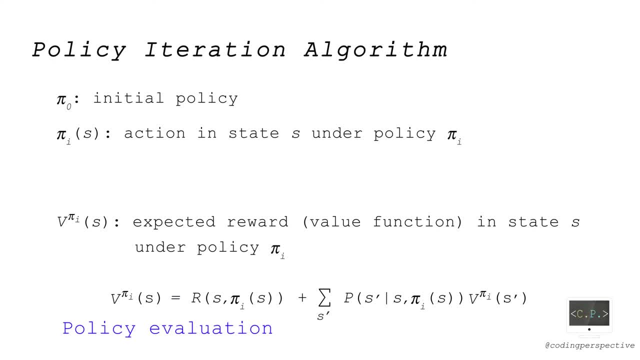 This is the second step and it's called policy evaluation, as we evaluate the current policy, pi i. In the last step, we improve our current policy by using v, pi, i. Basically, pi i plus 1 s is equal to arcmax of this expression. Again, the first part of the 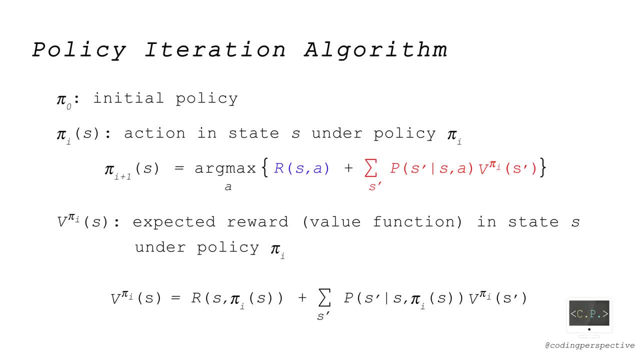 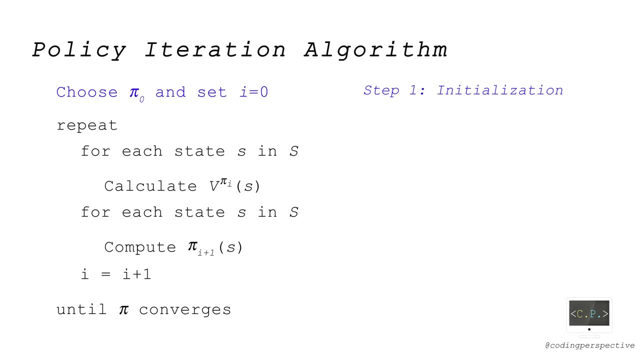 summation is the intermediate reward and the second part is the expected future reward. Until pi i is equal to pi i plus 1, we iterate step 2 and 3.. So we can summarize the policy iteration algorithm as you see. In step 1, we choose a policy, pi 0- and set i to 0. 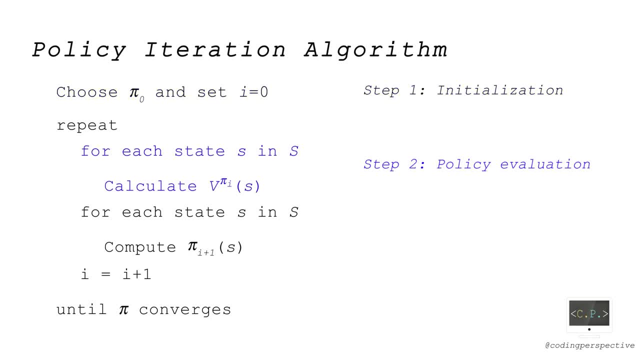 Then, at any iteration i, we calculate the current policy pi i. We calculate the value functions v, pi i for each state s under policy pi i by solving some set of linear equations. This is the policy evaluation step. After calculating these value functions, we compute pi i plus 1 s for each state s. 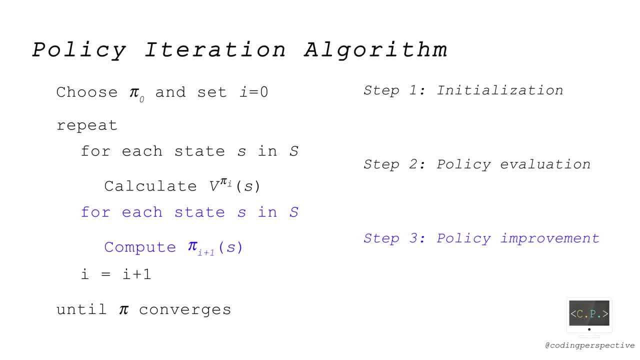 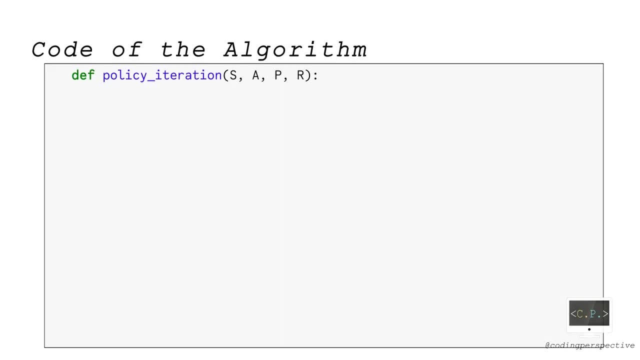 by using v, pi, i, And this is the policy improvement step. We repeat these two steps until policy pi converges. Now let's code this algorithm in Python by writing a function called policy iteration. The input of this function is the set of states s as a list. 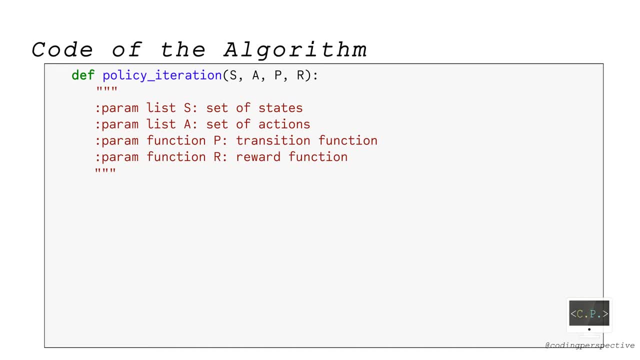 the set of actions, a as a list, the transition function p as a function and lastly, the reward function, r as a function. These inputs are totally problem-specific. I will later define them for a specific example. In the algorithm we first initialize policy dictionary by setting its value. 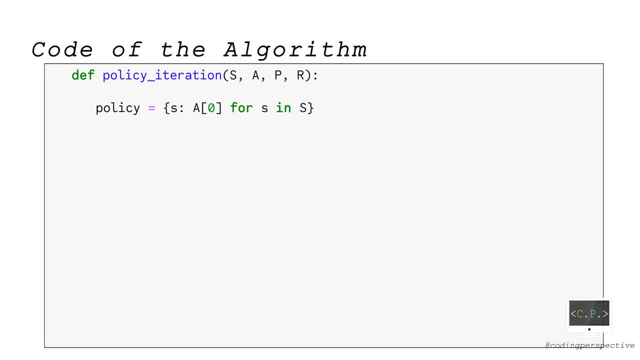 to some arbitrary feasible action for each state s. Here I choose s I choose to set them to the first element of action, set a. Then we have a while loop with a certain true condition. We will terminate it by using break once our termination condition. 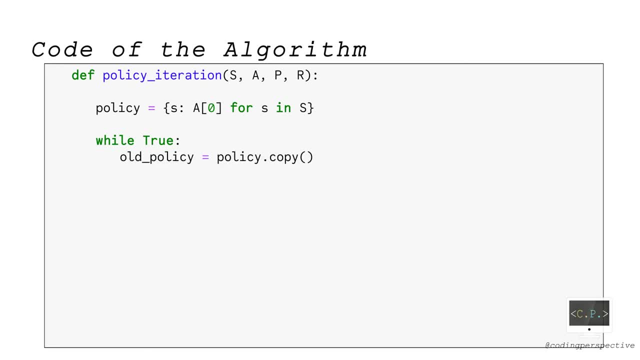 convergence of the policy is satisfied. Since we will update the policy at each iteration, I define a variable called oldPolicy to store the policy at the previous iteration. We can initialize it as a copy of the variable policy. The policy remains the same by comparing the variable oldPolicy with the variable policy. 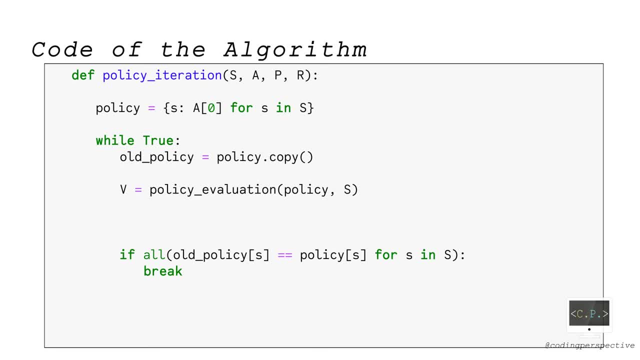 To update the policy at an iteration. we first calculate the value functions under the current policy. Here I use a function called policyEvaluation. This function takes the current policy along with the set of states s as inputs and then returns the value function under this policy as an output. 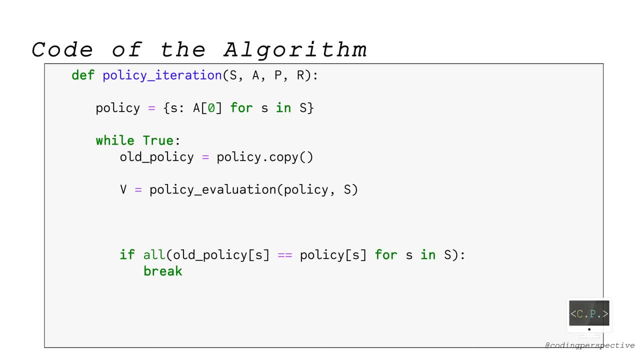 It is the policyEvaluation step of the algorithm. I will show how we can write this function in a bit. After calculating the value functions, we update our current policy by using a function called policyImprovement. Different than the function policyEvaluation, it takes the value functions together with 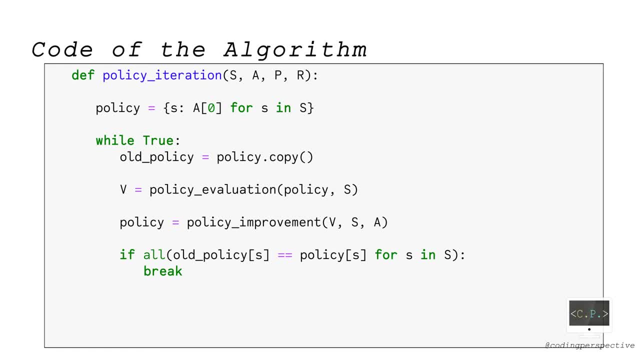 the set of states s and the set of actions a, as inputs and returns the updated policy as an output. This is the policy improvement step of the algorithm. If it is the same with the one in the previous iteration, we break the loop. Finally, we return policy as an output. 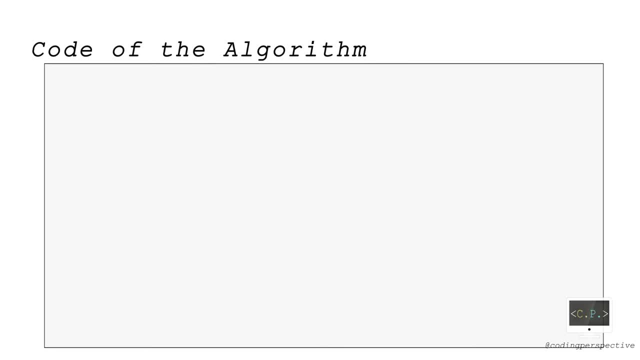 To complete the implementation of the policy iteration algorithm. now I will show how we can define policyEvaluation and policyImprovement functions. In policyEvaluation function the idea is updating the value functions under a given policy until they converge. For that we first initialize the value functions as a dictionary called v. 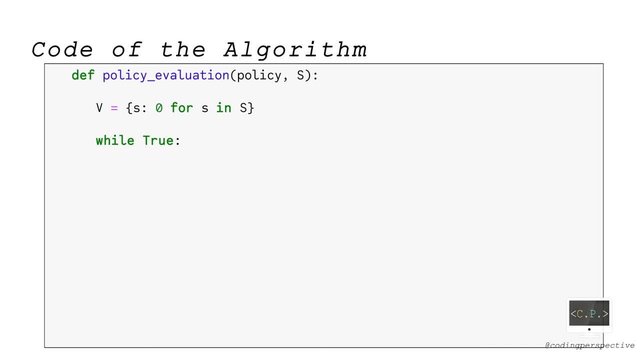 Then we have a while loop with a certain true condition. In this loop, we first create a copy of variable v called oldv. We use this loop to create a new variable called oldv. In this loop, we first create a copy of variable v called oldv.